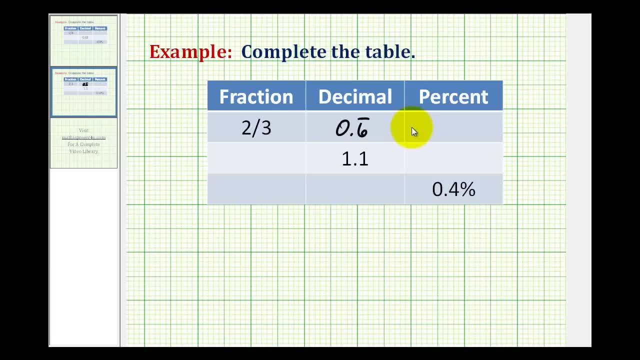 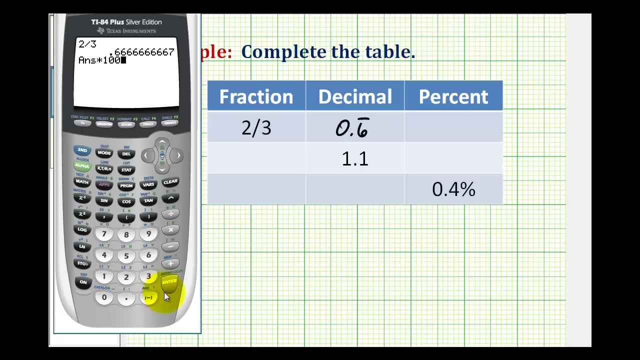 we multiply by one hundred and then add a percent symbol. So with the decimal value in the calculator we can just multiply this by one hundred. So as a percentage this would be sixty-six point six repeating, or sixty-six and two-thirds percent. Notice, multiplying by one hundred is the same as 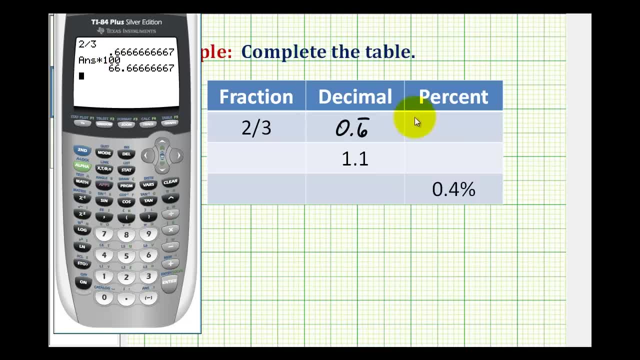 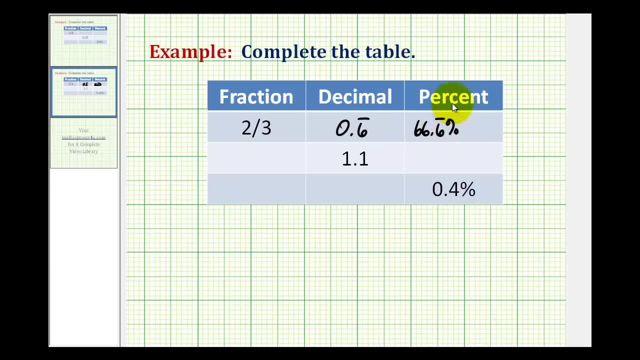 moving the decimal point two places to the right. So again we can write this two ways. We can write this as sixty-six point six percent, with the six repeating, or sixty-six and two-thirds percent. In the second row we want to write the decimal one point one, or one and one-tenth. 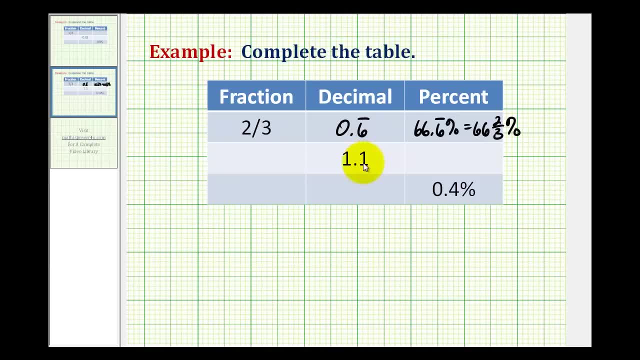 as a percentage and a fraction, So we can convert this to a percentage. in the same way, we converted point six, repeating, to a percentage: Multiply by one hundred and then add the percent symbol, Which again is the same as moving the decimal point to the right two places. 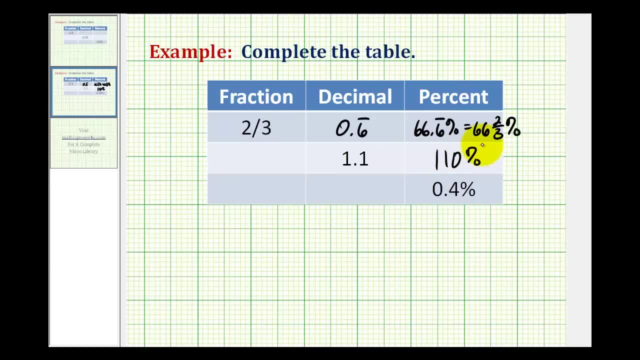 which would be one hundred ten percent. And then we know that a percentage is a number compared to one hundred, So the fraction would be one hundred ten over one hundred. And to simplify this we should recognize there's a common factor of ten, So we can divide both the numerator and denominator by two. 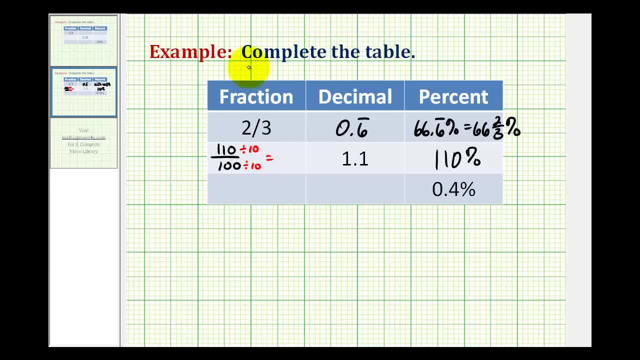 Divide by ten, which will give us a simplified fraction of eleven-tenths, And for the last row we have zero point four percent. We want to write this as a fraction and a decimal, So, as we said a moment ago, a percentage is a number compared to one hundred. 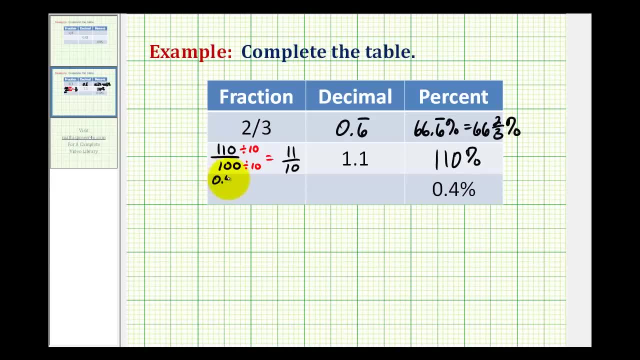 So written as a fraction, this would be zero point four over one hundred. But we can't leave a fraction in this form because we don't want to have a decimal inside a fraction. So if we take our current fraction and multiply the numerator and denominator by ten, 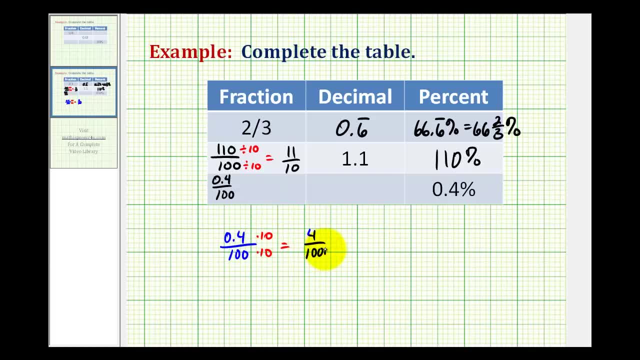 we would have four over a thousand. But now this can be simplified. They both have a common factor of four. Four divided by four is equal to one, And one thousand divided by four is equal to two hundred fifty. So the simplified fraction form would be one.